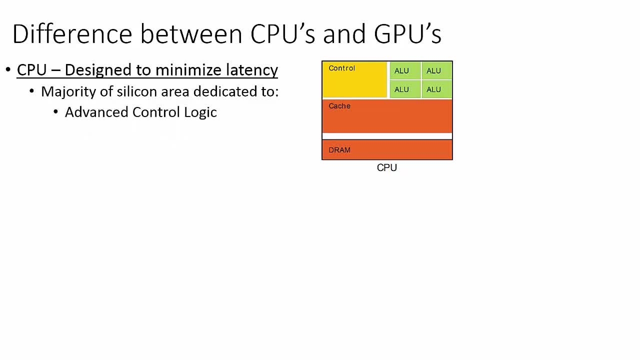 very fast on just a few tasks. To achieve this latency, the majority of the CPU area is dedicated to very sophisticated control logic and on-chip cache. This design works extremely well for very general purpose programs such as running operating systems system. Whereas CPUs are designed to minimize latency, GPUs are designed specifically to maximize. 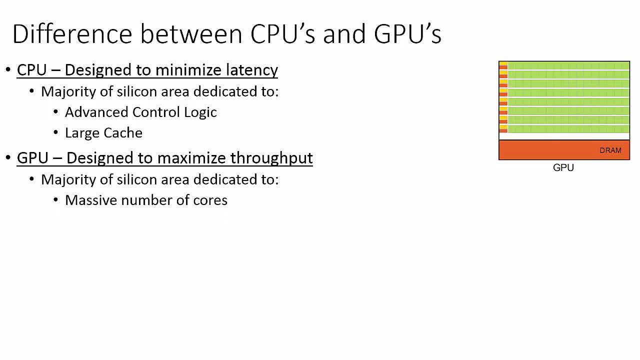 computational throughput. This design is characterized by dedicating the majority of the silicon's area to a massive number of arithmetic logic units, which NVIDIA calls CUDA cores. More specifically, the GPU is well-suited to address problems that can be expressed as data-parallel computations, where the same program is executed on many data elements. 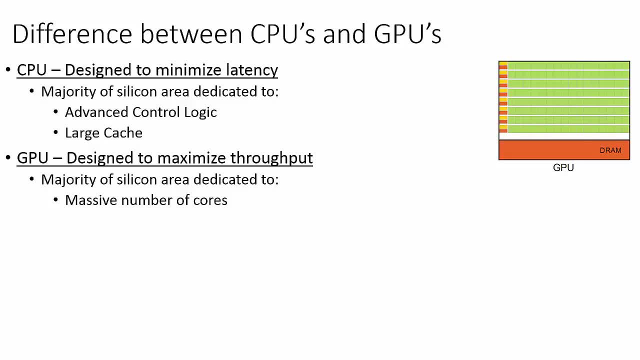 in parallel. Because the same program is executed for each data element, there is a lower requirement for sophisticated control logic, and because it is executed on many data elements, the memory access latency can be hidden with calculations instead of big caches In order to properly utilize a GPU. the parts of the program that can 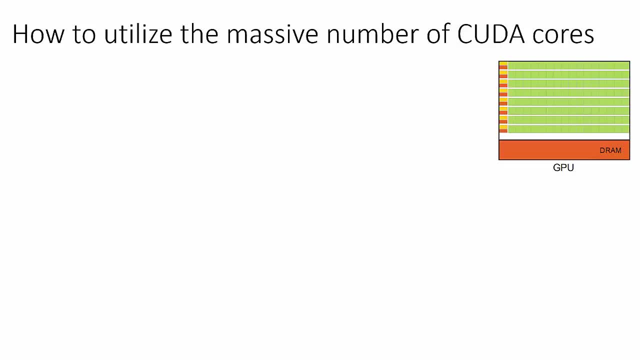 be parallelized must be decomposed into a large number of threads that can run concurrently. In CUDA, these threads are defined by special functions called kernels. A kernel is simply a function that is executed on the GPU. The execution of kernel is called launching a kernel. 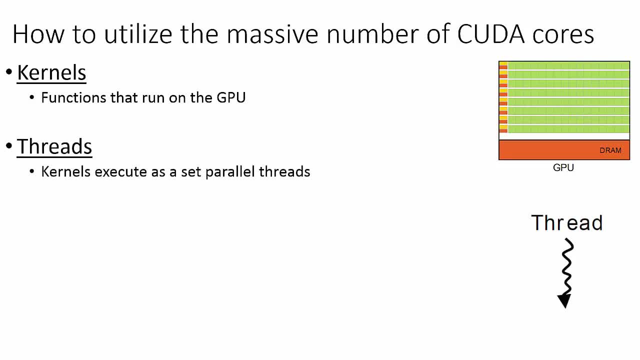 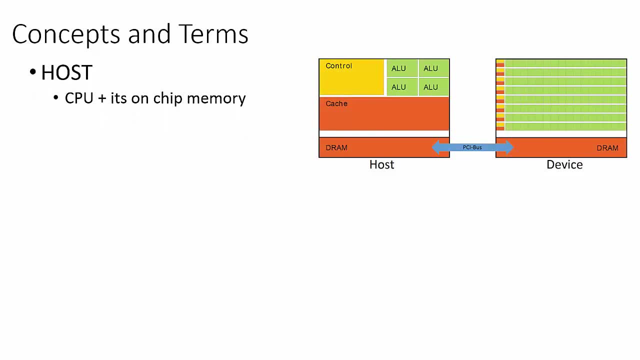 When we launch a kernel, the kernel is executed as a set of threads. Each thread is mapped to a single CUDA core on the GPU. The two main pieces of hardware in the CUDA programming model are the CPU and the GPU, each with their own dedicated memory region. 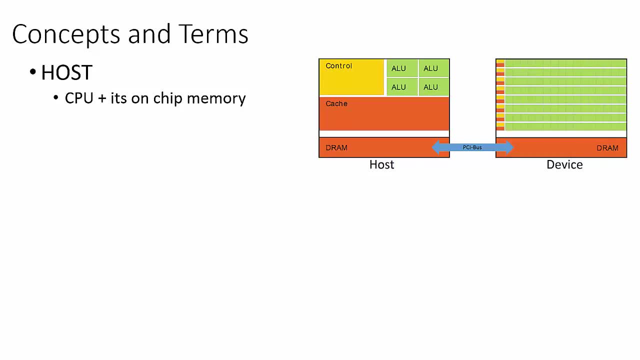 The CPU, together with the computer's RAM, is referred to as the host. Similarly, the GPU, together with its own dedicated DRAM, is called the device. The CPU is very good at running serial programs. The problem with CPUs is if they run into a portion of code that is massively parallel. 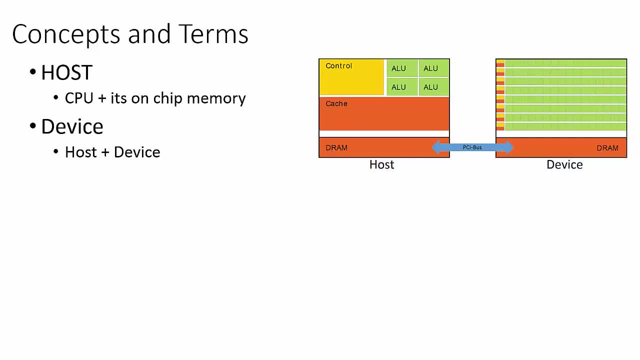 this part of the program will likely cause a bottleneck in the flow of the program, since CPUs are just not designed for massively parallel throughput. Since GPUs are very good at running a part of a program that is very parallel, we want to offload these massively parallel portions of the code onto the GPU. 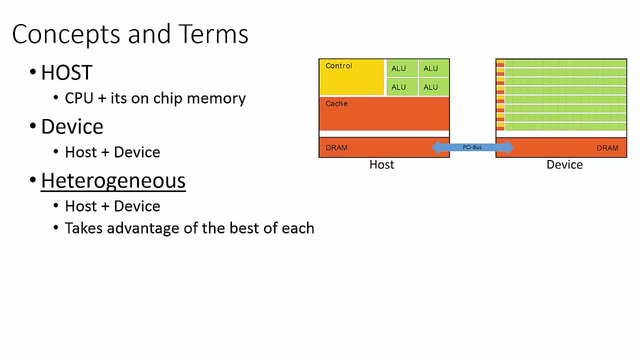 Using the host and device together is termed heterogeneous parallel programming. This is where CUDA comes in. CUDA is the heterogeneous parallel programming. This is where CUDA comes in. CUDA is the heterogeneous parallel programming language designed specifically for NVIDIA GPUs. CUDA is simply C with a set of extensions that allows for the host and device to work. 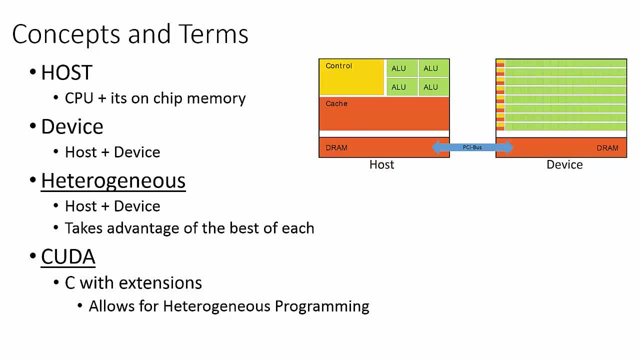 together. In the CUDA programming model, the host is in control of the program. For the most part, a CUDA program will run just like a traditional piece of software would on the CPU. Whenever we run into a portion of code that can be massively parallelized, we will pass. 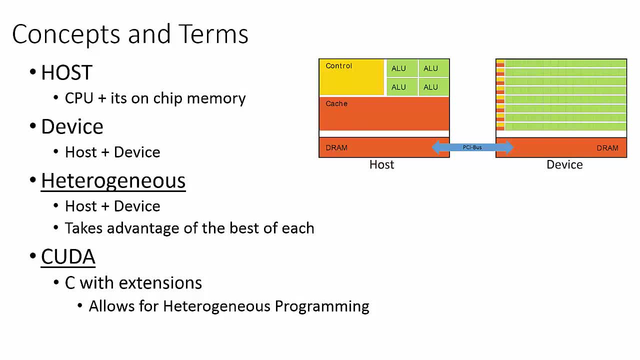 on that portion of code to the device. The hosts and devices talk to each other over the PCI Express Bus, which is very slow relative to the host and device, So the cost of exchanging data between the host and device is very expensive. Therefore, the only portions of the code that we want to execute on the device are the parts: 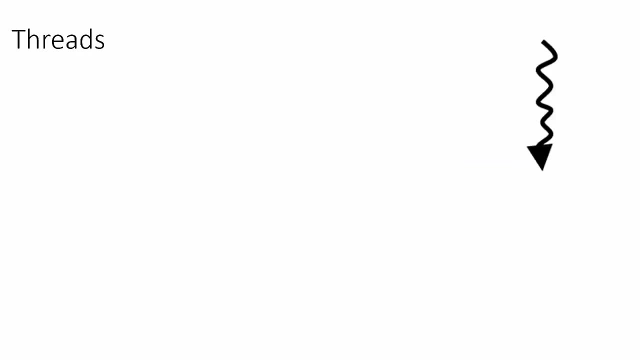 that are massively parallel. The most common reason for the PCI Express Bus to work is because the PCI Express Bus is the most complex process. It needs to run on the PCI Express Bus. This is where we get the most data. Let's take a closer look at the concept of the PCI Express Bus. 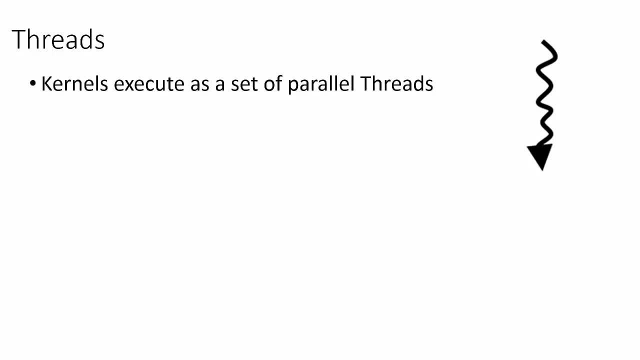 Let's take a closer look at the concept of the PCI Express Bus, the CUDA thread. To utilize the massive number of cores on the GPU, we want to execute CUDA kernels as a very large number of threads. The GPU is designed to execute each kernel as thousands. 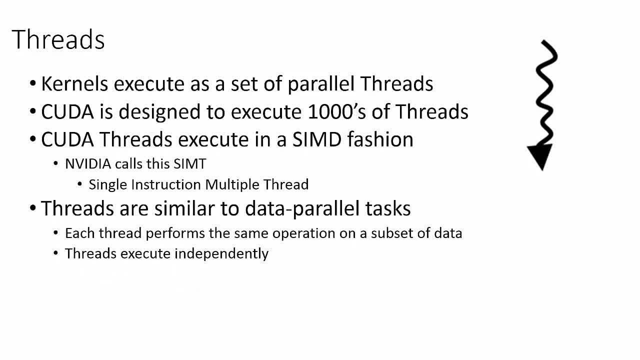 or even millions of threads. CUDA threads execute in a single instruction multiple data fashion, commonly termed SIMD in the computer architecture literature. That is, each thread executes the same instruction but on a separate piece of data. The exact manner in which threads execute is: 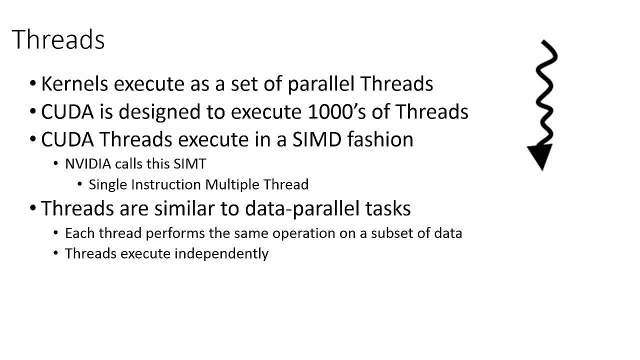 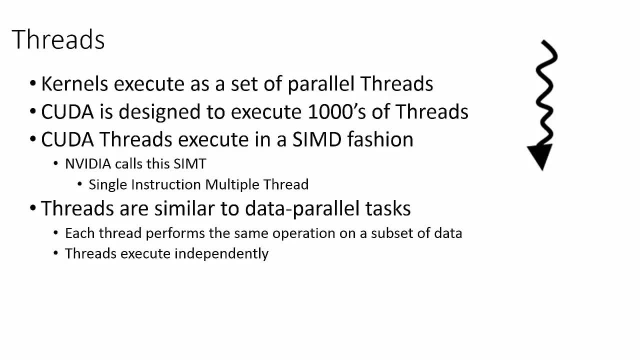 really important here, but these terms are thrown around in the CUDA literature, so just think of these terms as having the same meaning. Another thing to note is that threads do not all execute at the same rate, Even though each thread is performing the same operation: the set of data being computed. 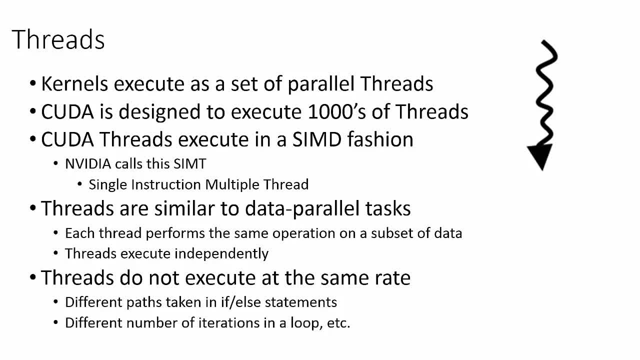 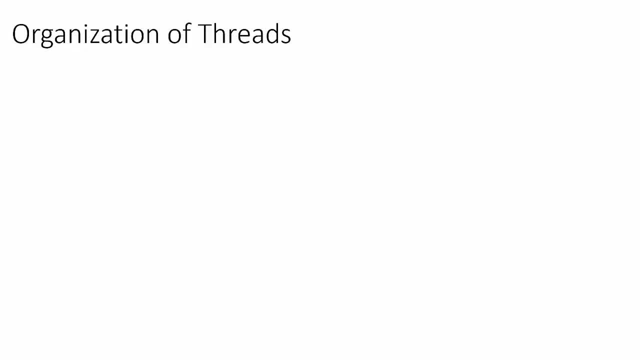 on in each thread is generally different, which can give rise to threads from the same kernel executing at different rates. In order to organize how threads are mapped to cores on the GPU, CUDA has a hierarchy of threads. Now, this is one of the most important concepts in CUDA's programming. 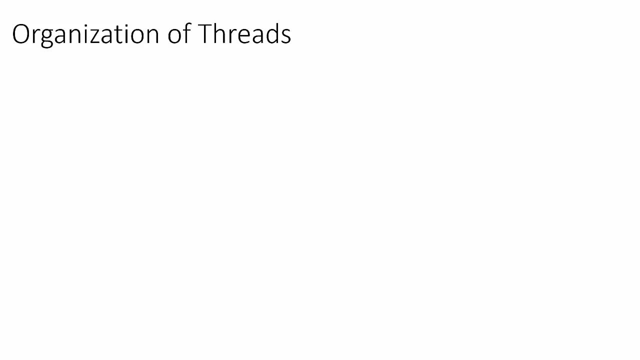 model. There are three levels in the hierarchy, which we will discuss now. At the lowest level of the hierarchy we have individual threads. We've already seen the thread which is the execution of a kernel on a single piece of data. Each thread gets mapped to one CUDA core on the GPU. when the 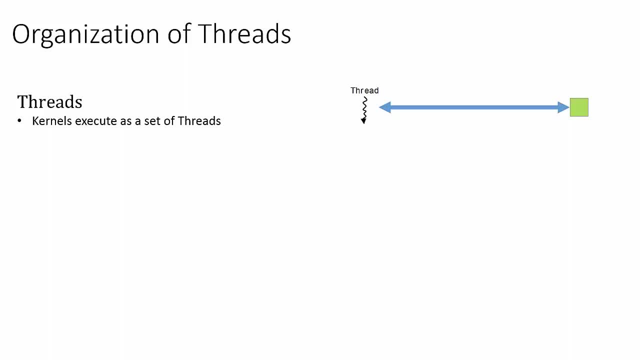 kernel is launched. In the next level of the hierarchy, we have a structure called a block. Sets of threads are grouped into blocks. When the kernel is launched, the blocks get mapped onto corresponding sets of CUDA cores, which will be covered in the following lecture. At the highest, 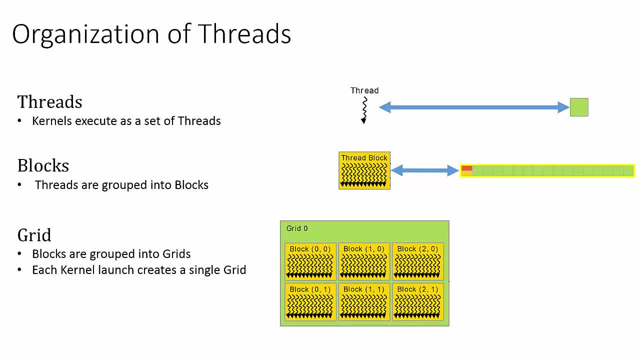 level of the CUDA hierarchy, we have grids. The entire kernel launch is executed as one grid which is mapped onto the entire GPU and its memory. In summary, one kernel launch executes as one grid which is mapped onto the entire device. To keep terms in order, it may be helpful to think of threads as elements of blocks and blocks as 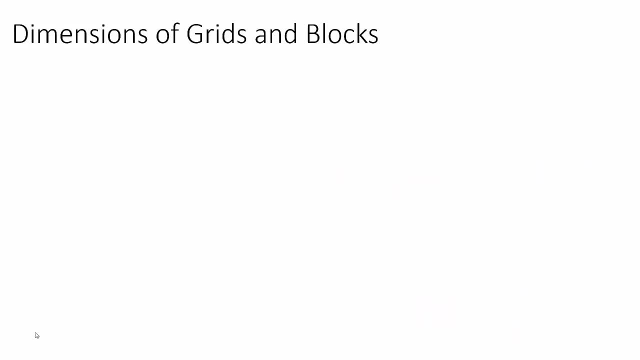 elements of grids. So each grid is composed of a set of blocks, which are organized into either a 1D, a 2D or a 3D structure. In this example, the block structure is composed of a 3 by 2 grid, So there are three blocks in the X dimension and two blocks in the Y dimension, giving us a total of six blocks in this grid. Analogously, blocks are composed of threads, which are also organized into either a 1D, a 2D or a 3D structure.